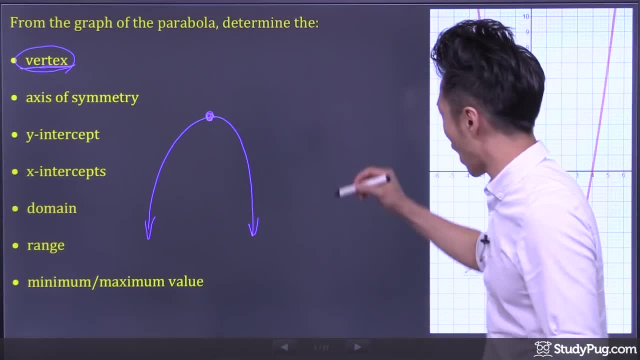 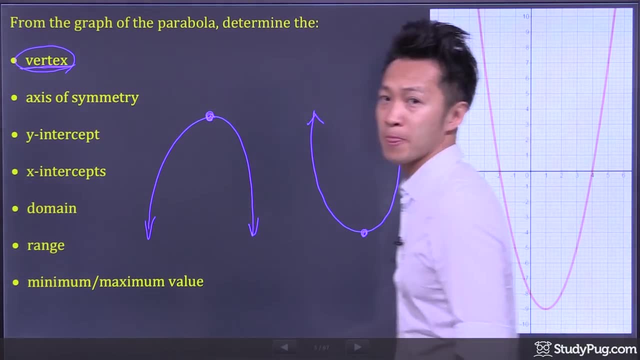 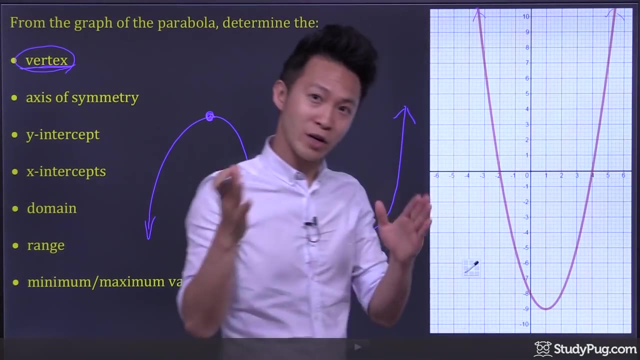 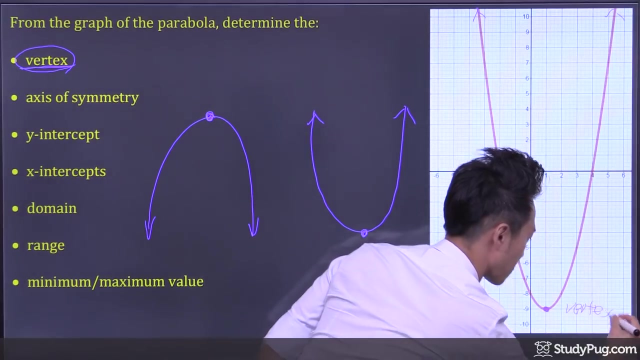 the highest point. Now for a parabola opening up, the vertex is the lowest point. So in this case we have a parabola opening up, So the vertex is the lowest point right here, sitting at x equals 1,. y equals 2,, 3,, 4,, 5,, 6,, 7,, 8,, 9,, 10,, 11,, 12,, 13,, 14,, 15,, 16,, 17,. 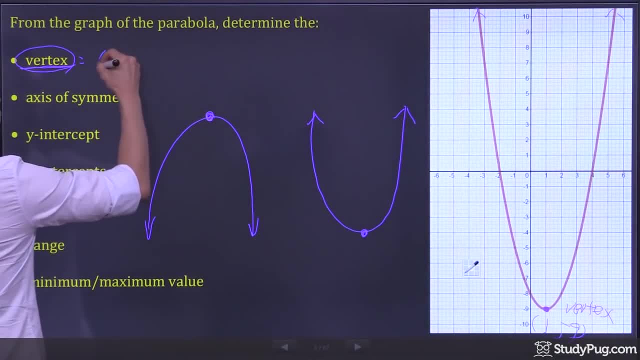 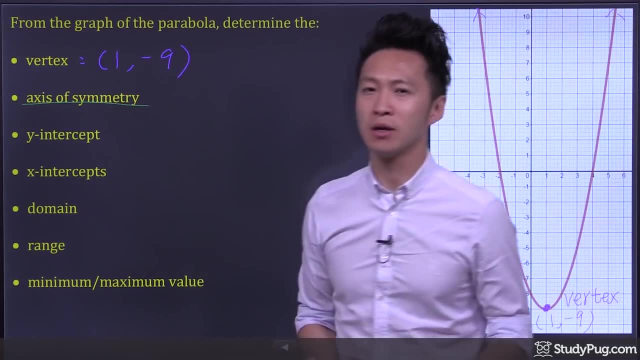 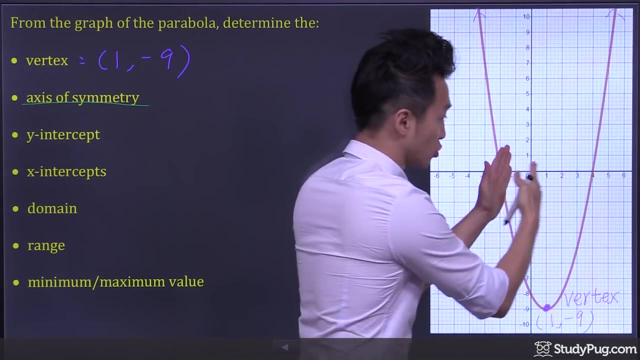 18,, 19,, 20.. So the vertex is at 1 and negative 9.. Next, axis of symmetry. The axis of symmetry of a quadratic function is a vertical line that divides the parabola into two equal halves, like this: 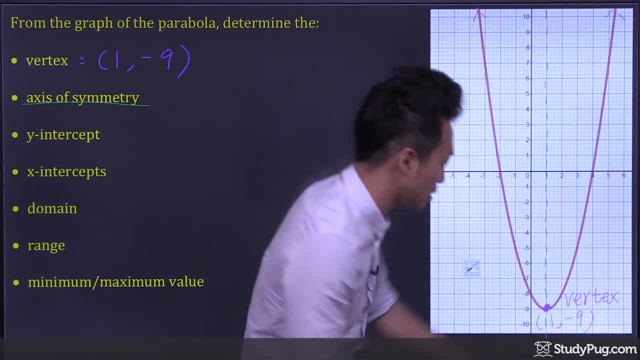 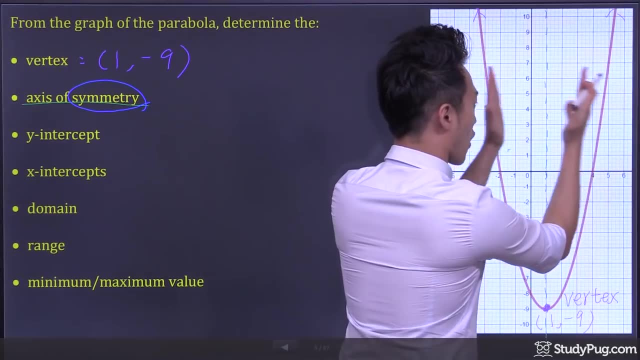 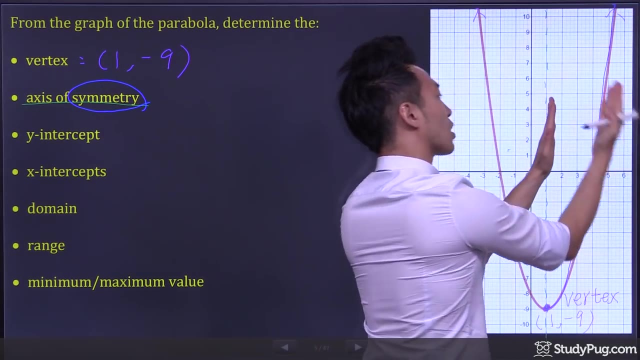 And the axis of symmetry must always pass through the vertex. The symmetry behavior can be best understood when we fold the parabola in half along the axis of symmetry. Then the right half of the parabola will completely overlap the left half of the parabola Can. 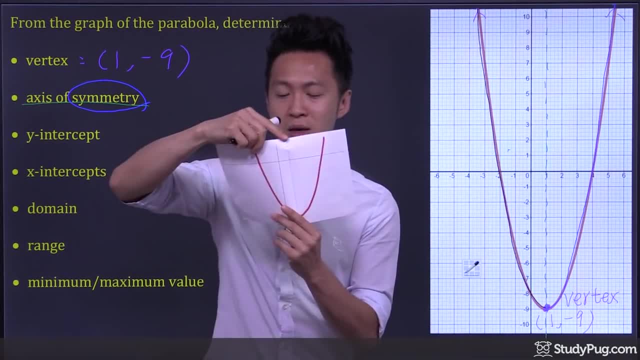 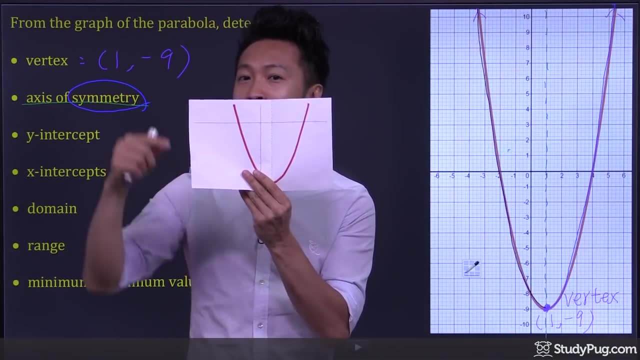 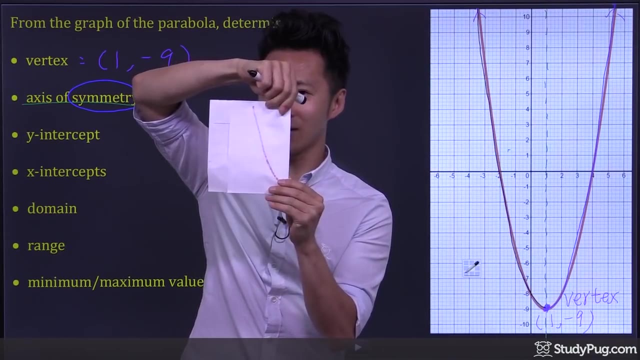 you see that? Let me show you Here. we have a parabola just like this one, And then we have an axis of symmetry that runs down the middle of the parabola. Now I'm going to fold the graph along the axis of symmetry. Can you see that? The two halves of the parabola. 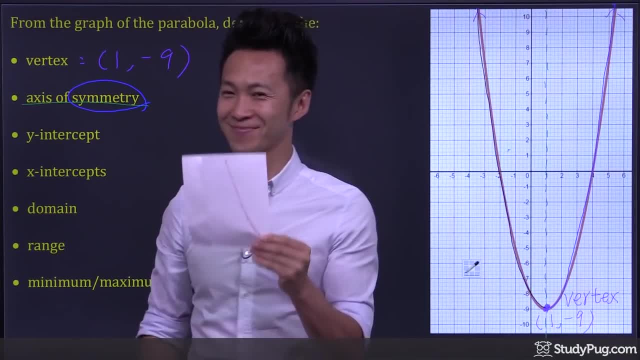 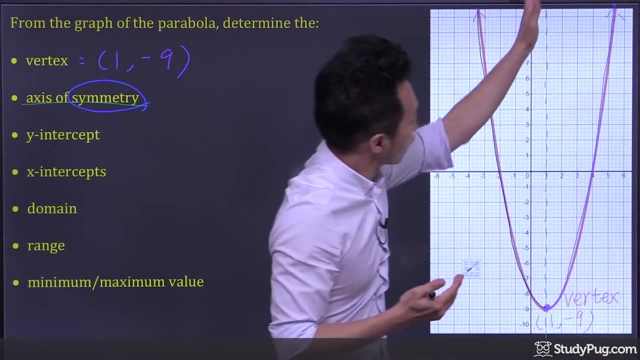 completely overlap each other. Yeah, Cool. Now let's determine the equation of the axis of symmetry For a vertical line that passes through: x equals 1, y equals 2,, 3,, 4,, 5,, 6,, 7,, 8,, 9,, 10,, 11,, 12,, 13,, 14,, 15,, 16,, 17,, 18,, 19,. 20,, 21,, 21,, 22,, 23,, 24,, 25,, 26,, 27,, 28,, 29,, 30.. Now let's look at the equation of the axis of symmetry. We're going to find the axis of symmetry and we're going to find out. 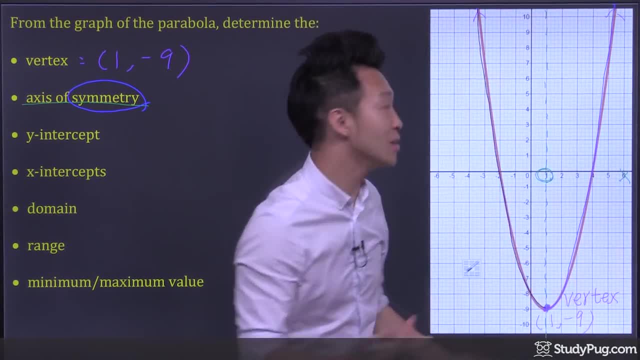 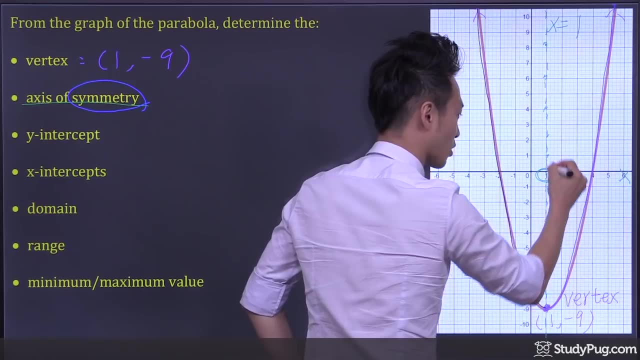 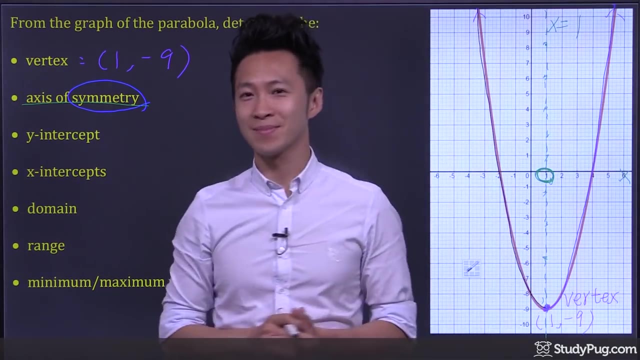 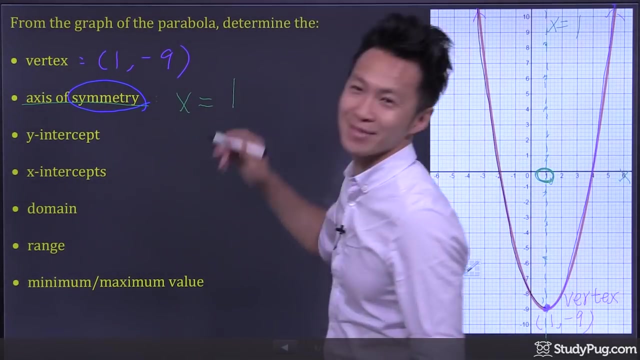 what the axis of symmetry is. We're going to find that x equals 1.. The equation of the line is simply x equals 1.. Because for every point on this vertical line, the x coordinate is always 1.. So in this case, the equation of the axis of symmetry is x equals 1.. Next, 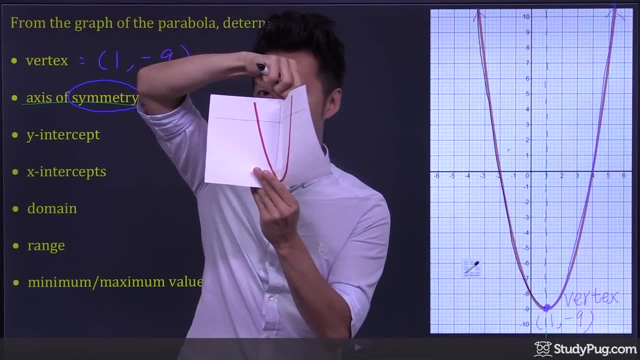 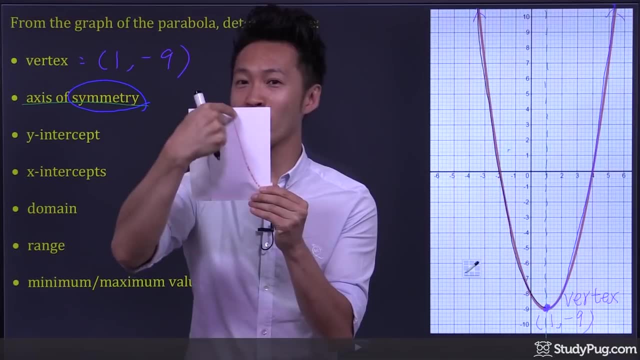 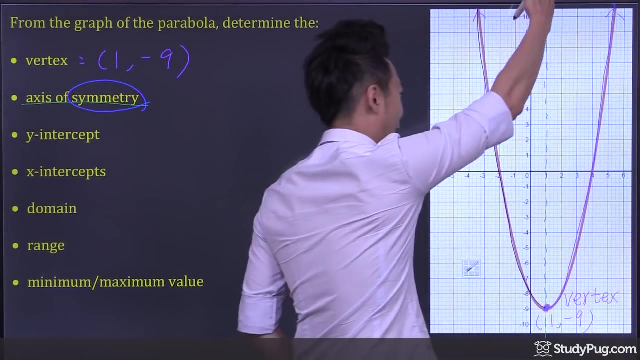 graph along the axis of symmetry. Can you see that The two halves of the parabola completely overlap each other? Yeah Cool, Now let's determine the equation of the axis of symmetry For a vertical line that passes through a vertical line that passes through a vertical. 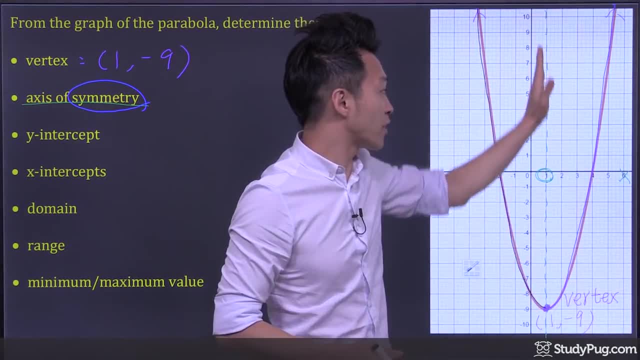 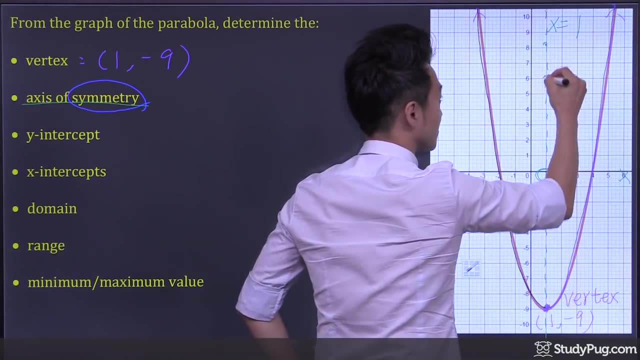 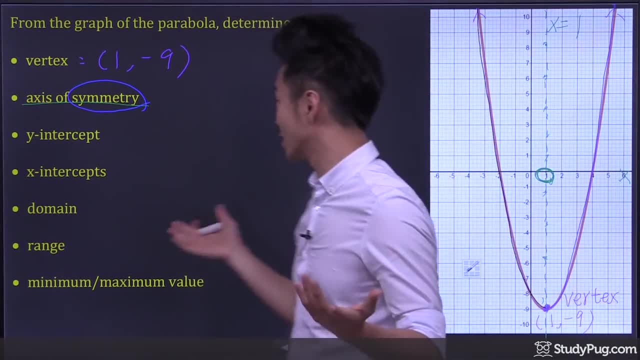 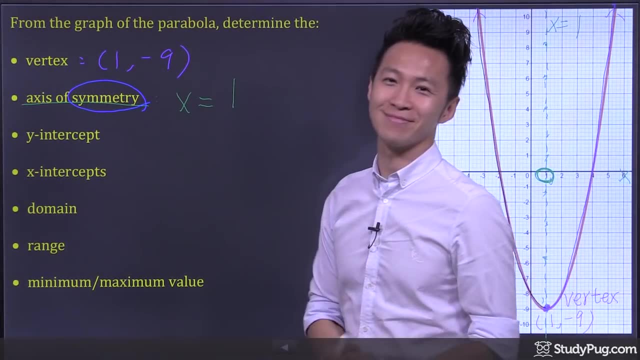 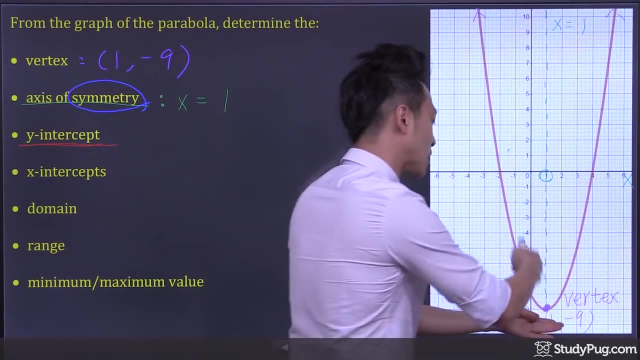 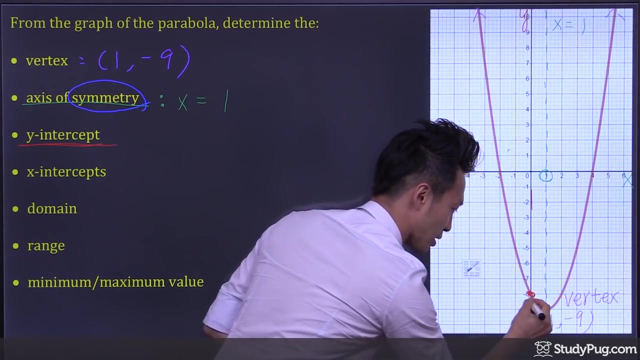 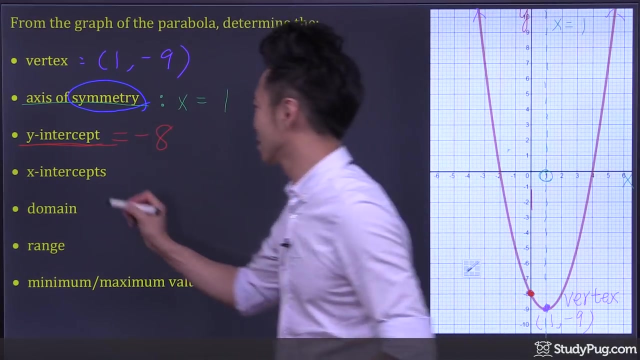 vertical line. the x coordinate is always 1.. So in this case the equation of the axis of symmetry is: x equals 1.. The y-intercept is the point where the parabola intersect the y-axis. So in this case that's right here And the y-intercept is negative 8.. Next, x-intercepts. The x-intercepts. 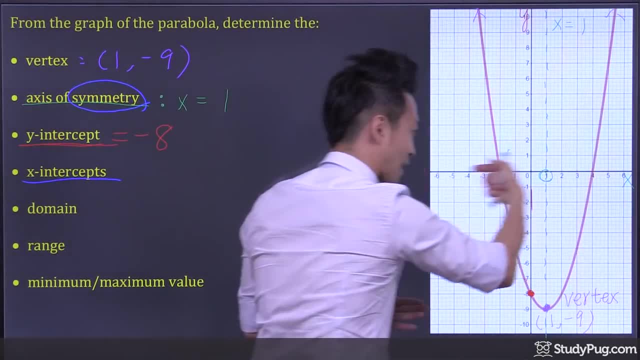 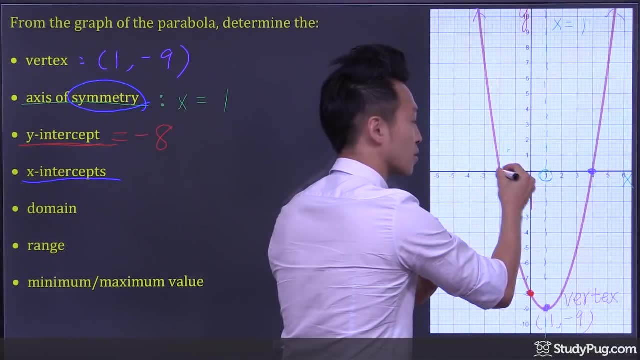 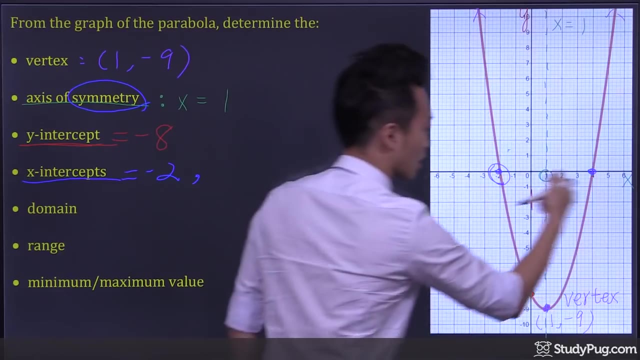 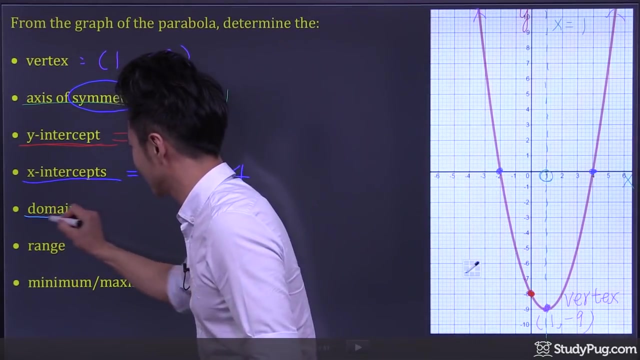 are the points where the parabola intersect the x-axis. So in this case the parabola intersects the x-axis at two points: One at x equals negative, 2. Another one at x equals 4.. Next domain: By definition, domain is the set of x values for which a function is. 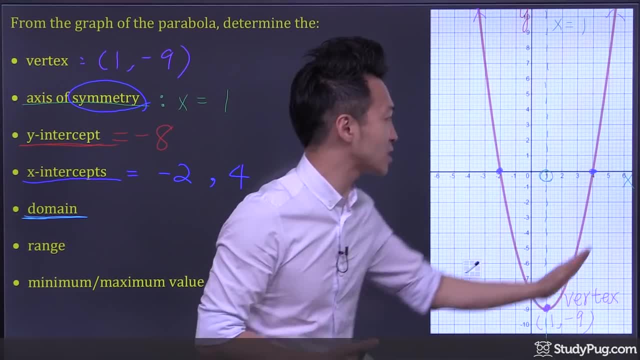 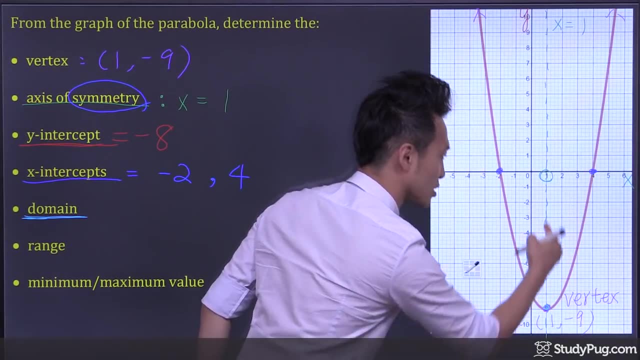 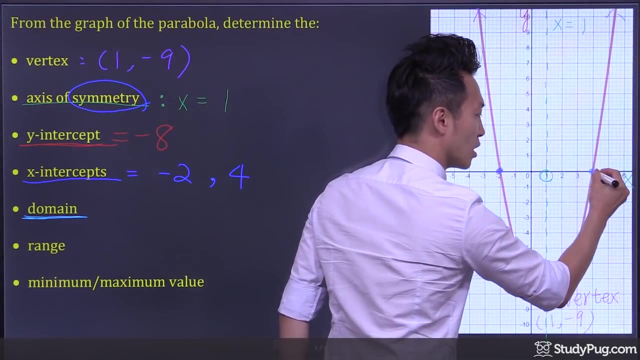 defined. So, as we can see, a parabola is defined for all x values. Let me show you This point: the x value is positive. 1. At this point, x value is positive. 2. At this point, x value is positive. 3. At this point, x value is positive. 4. At this. 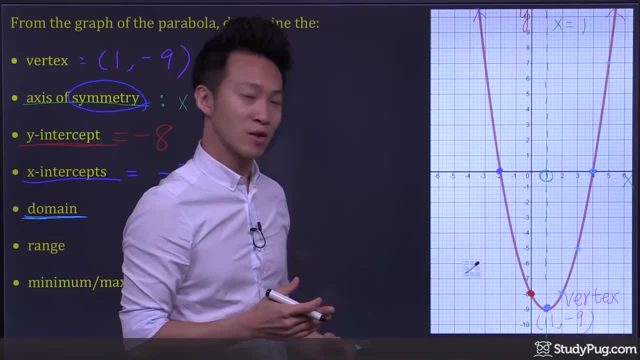 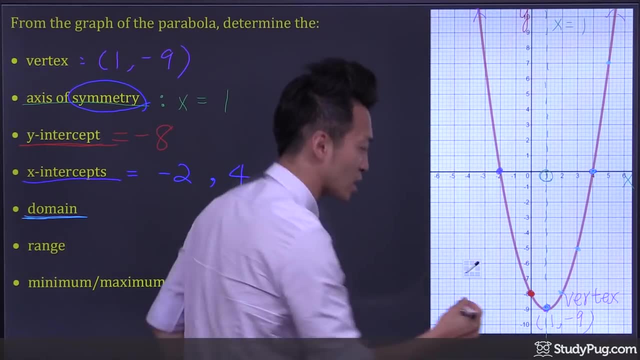 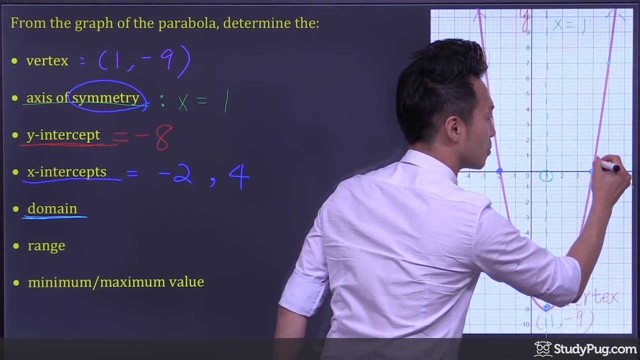 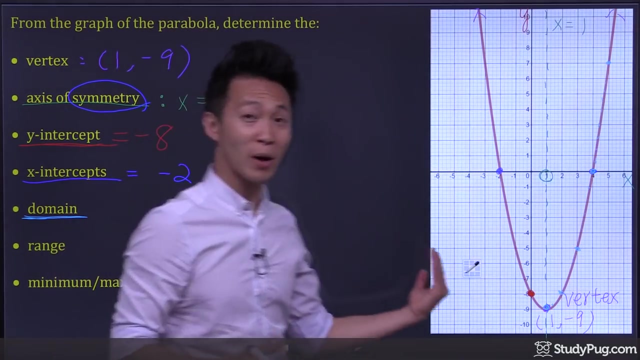 point: x value is positive 5. So a parabola is defined for all positive integers for x. Now, if you take any points in between, now see these points are all x values. So you can see that the x values are positive decimal numbers. right, Yeah, So a parabola can take. 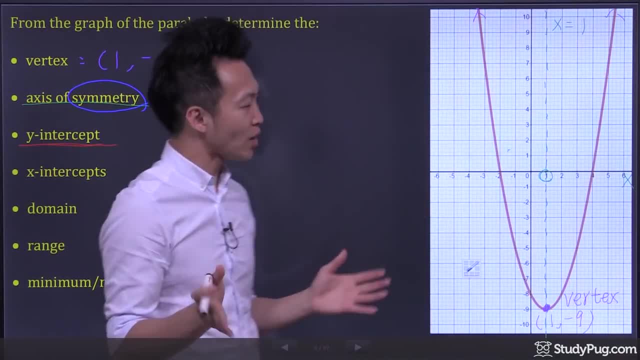 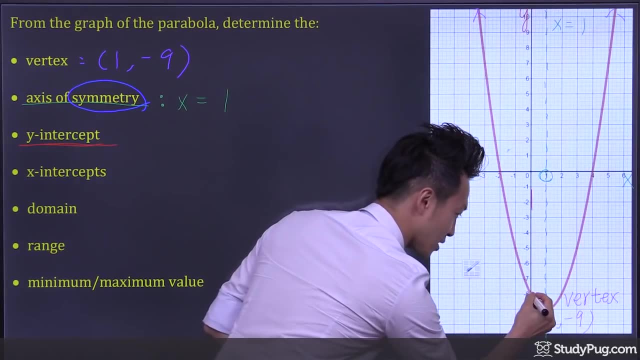 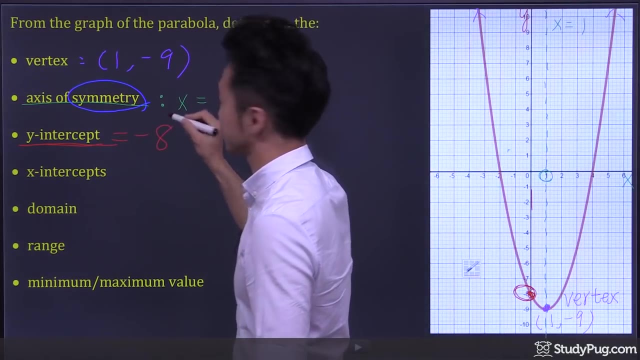 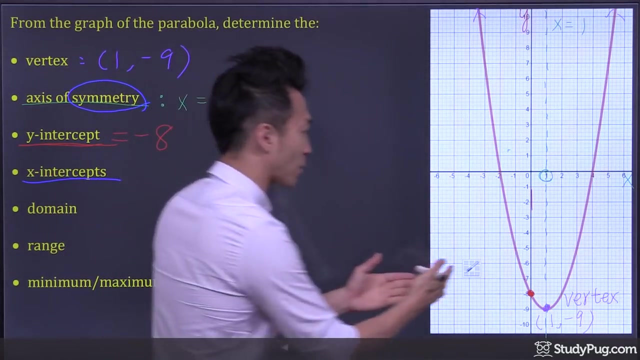 y equals 2. intercept: The y-intercept is the point where the parabola intersect the y-axis. So in this case that's right here And the y-intercept is negative. 8. Next, x intercepts: The x-intercepts are the points where the parabola intersect the x-axis. 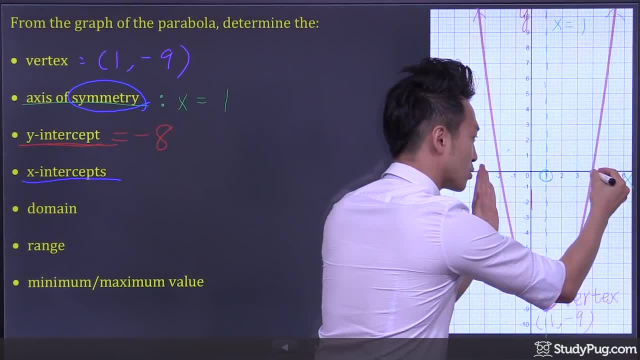 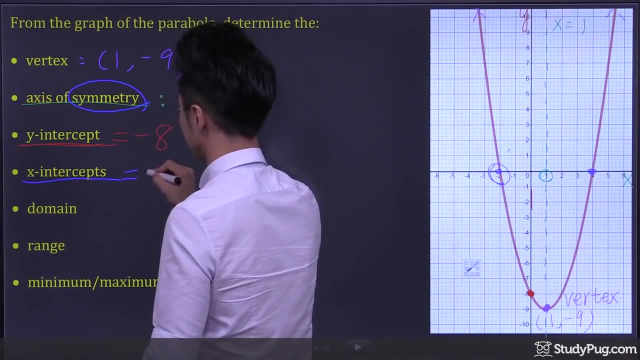 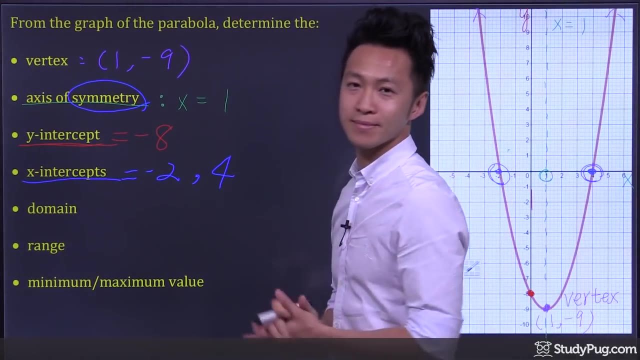 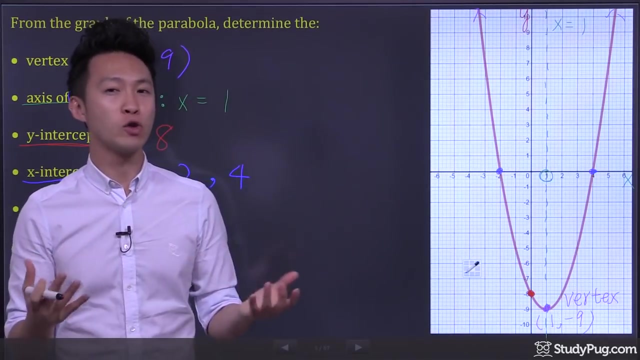 So in this case, the parabola intersects the x-axis at two points: One at x equals negative 2, another one at x equals 4.. Next domain: By definition, domain is the set of x values for which a function is defined. So, as we can see, a parabola is: 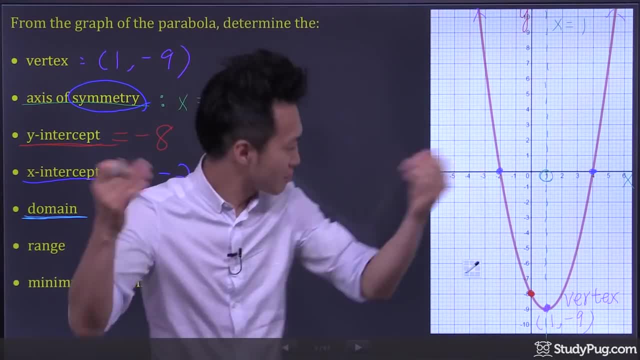 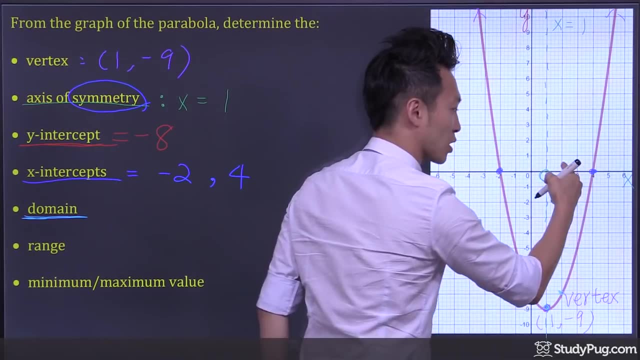 defined for x, All x values. Let me show you This point: the x value is positive. 1. This point x value is positive. 2. This point: x value is positive. 3. This point x value is positive. 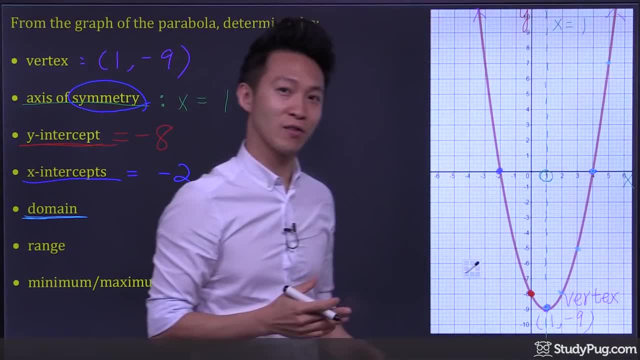 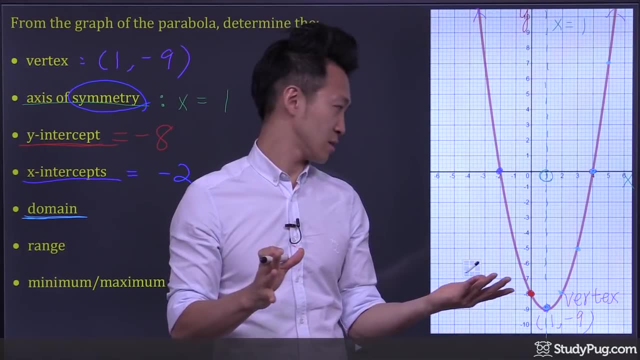 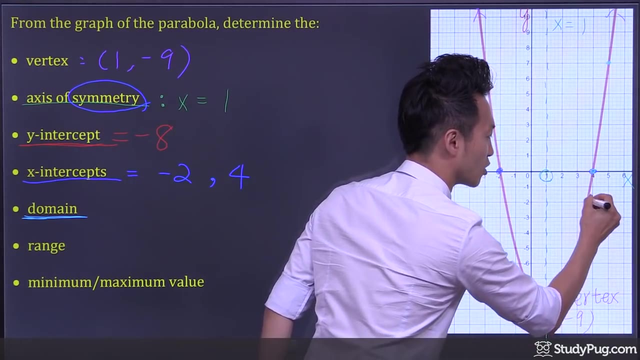 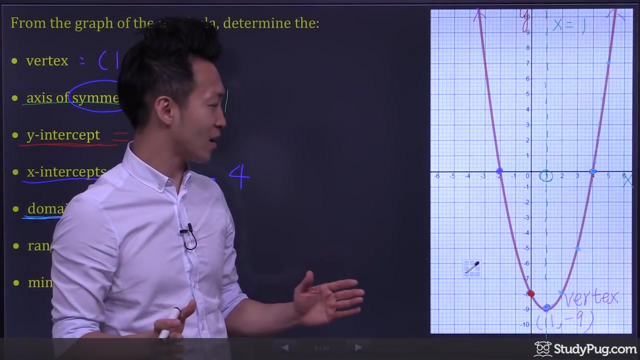 4. This point: x value is positive. 5. So a parabola is defined for all positive integers for x. Now, if you take any points in between, now see, In this point the x values are positive decimal numbers. right, Yeah, So a parabola. 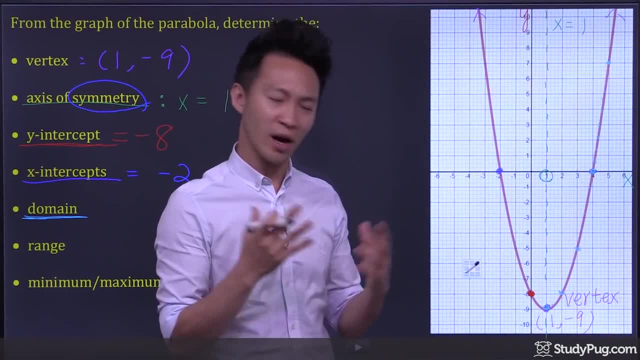 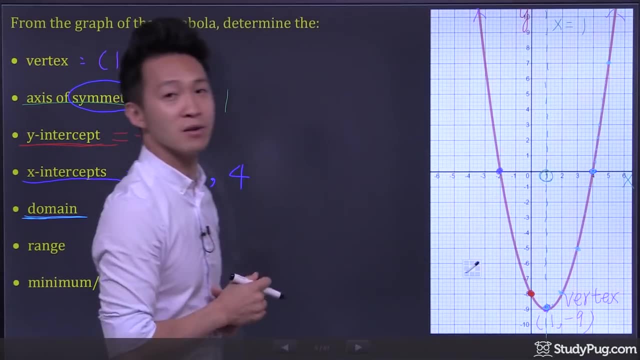 can take on any positive value for x. whether they are integers or they are decimal numbers, Parabola can take on any positive numbers for x. Now guess what Parabola can also take on any negative values for x. For example, this point: x value is negative 1.. Where this: 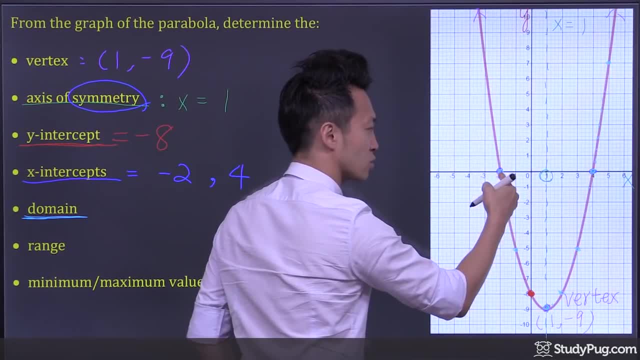 value is this points point where this positive values go by saying for x given for all revenues, and instead of this I plant x as negative, whether they are integers or if they: 1. This point x value is negative. 2. This point x value is negative. 3. See negative. 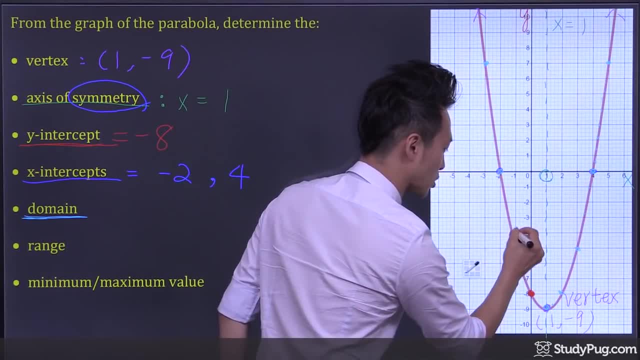 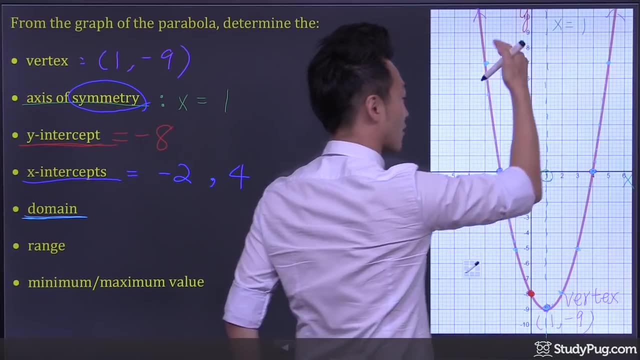 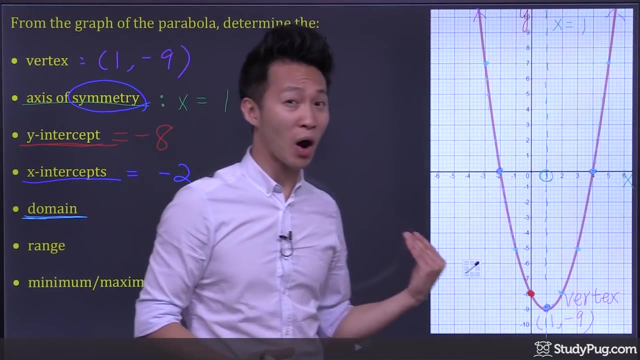 integers. Now for any points in between them, for any points between the negative integers, see this point. the x values are all negative decimal numbers. So, in conclusion, parabola can take on any positive values for x. Parabola can also. 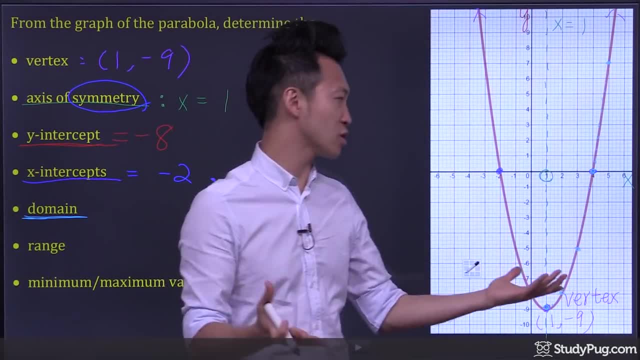 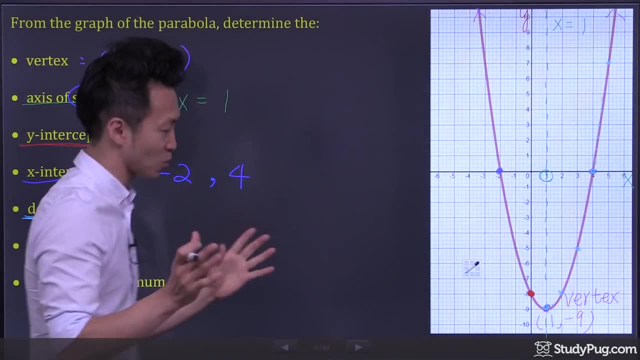 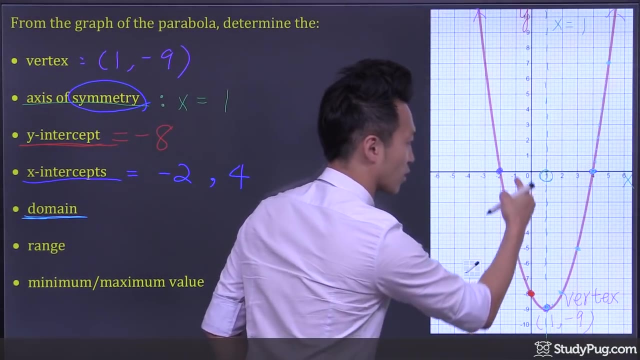 on any positive values for x. whether they are integers, whether they are decimal numbers, Parabola can take on any positive numbers for x. Now guess what? Parabola can also take on any negative values for x. For example, this point: x value is negative. 1. This point: 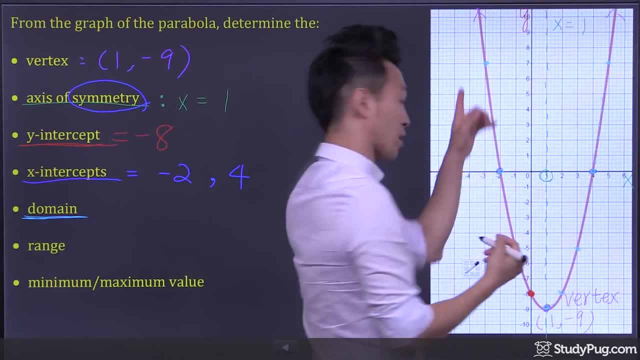 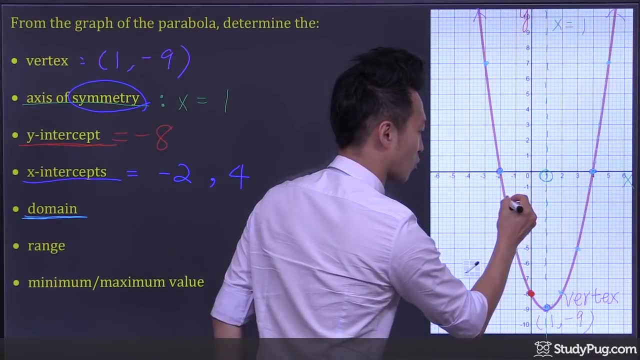 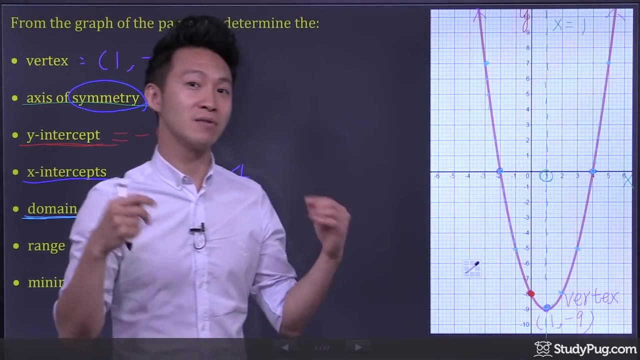 x value is negative. 2. This point x value is negative. 3. See negative integers Now for any points in between them, for any points between the negative integers, see this point. the x values are all negative decimal numbers. So, in conclusion, parabola can take on any. 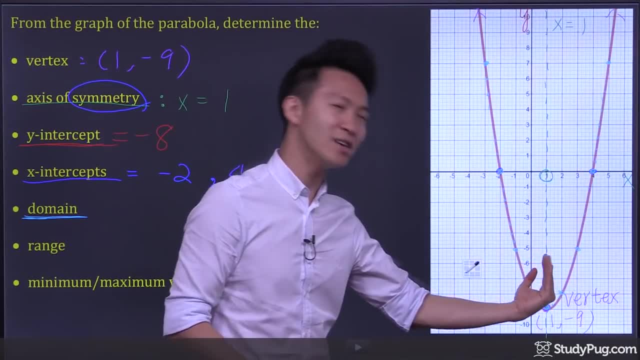 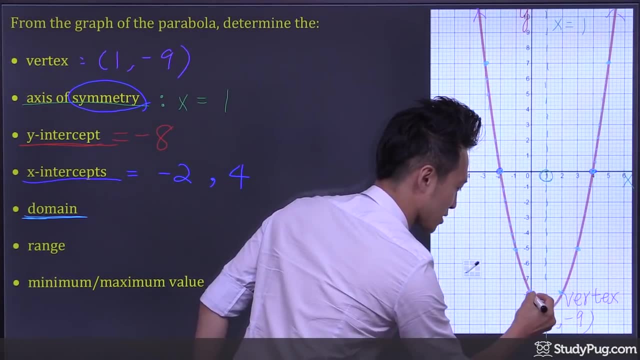 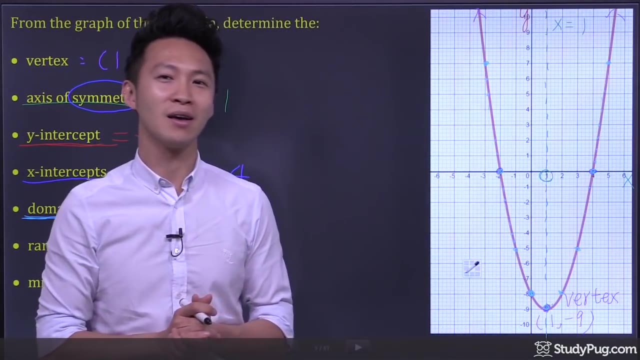 positive values for x. Parabola can also take on any negative values for x, And parabola can either take on 0 for x. That would be this point, See for the y-intercept. the x value is 0, right. 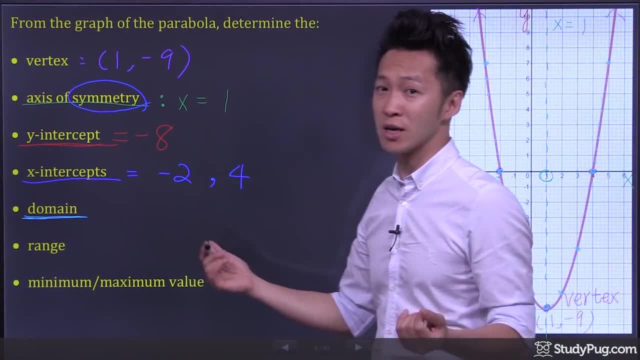 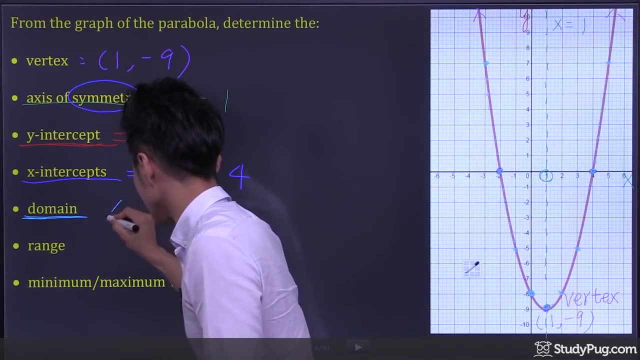 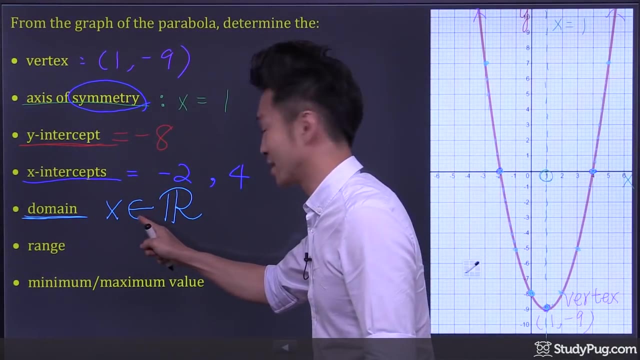 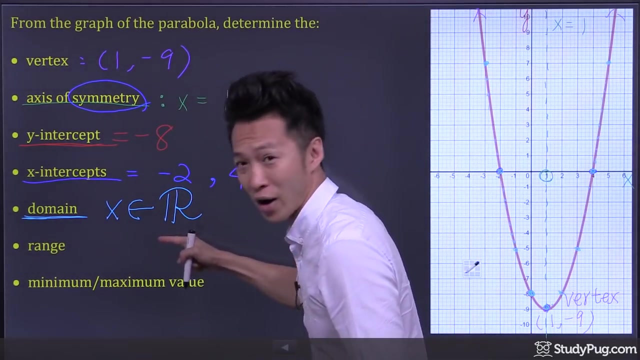 So therefore, the domain for a quadratic function is all real numbers And we write a mathematical notation like this: X is all real numbers, right? This symbol means is: And this symbol here represents- see this symbol here is a r with an extra bar- represents all real numbers. 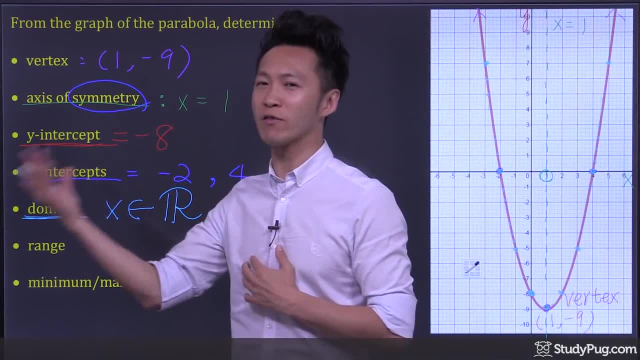 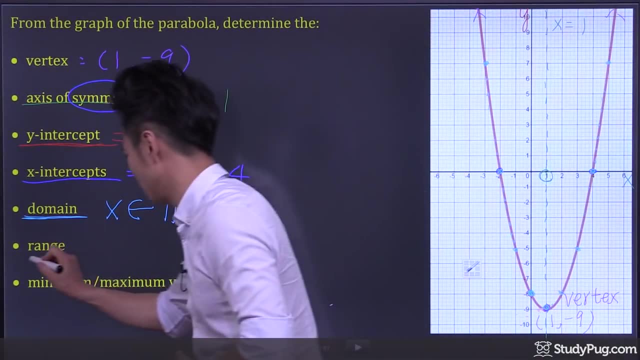 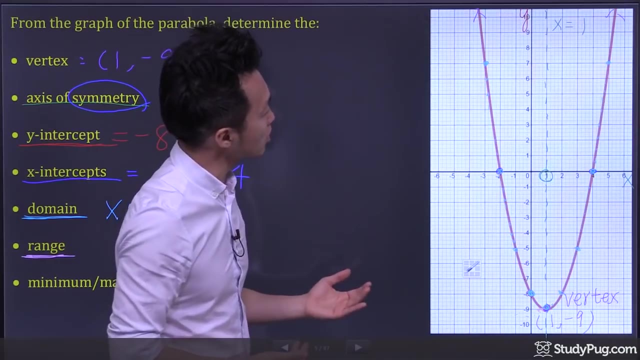 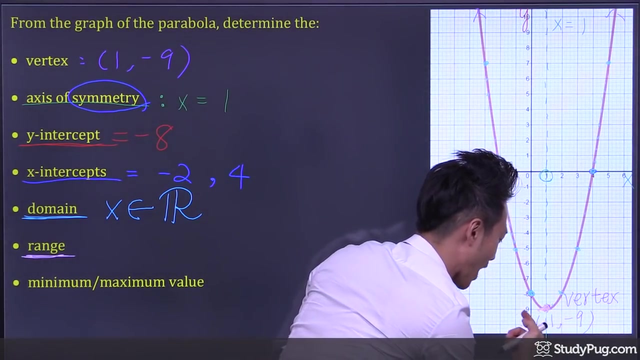 In fact the domain for any quadratic function is always: x is all real numbers. Next range: By definition, range is the set of y values for which a function is defined. So here the parabola only go as low as right here, where the y value is negative, 9.. However, 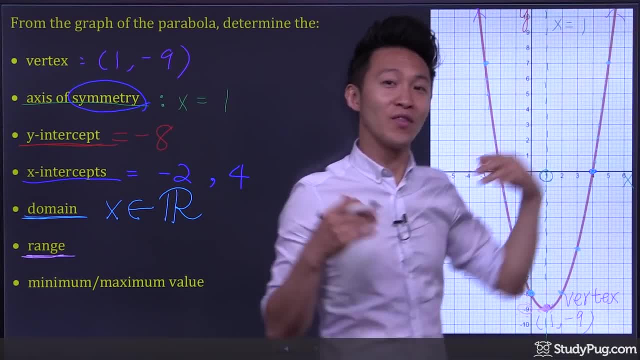 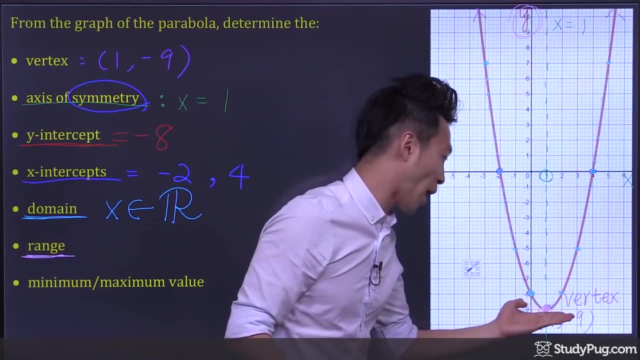 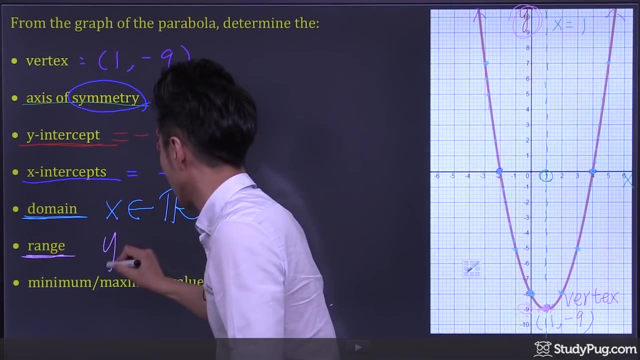 it will go as high as it likes. And therefore we say: the range range talks about y, right, So the range is y must be negative 9 and y must be negative 9.. Okay, And anything above. So the range is y is greater than or equal to negative 9.. Does this parabola 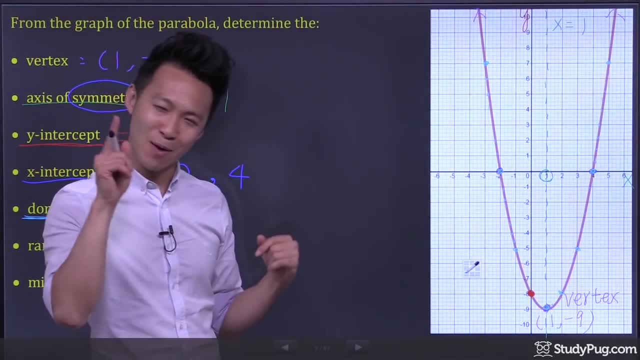 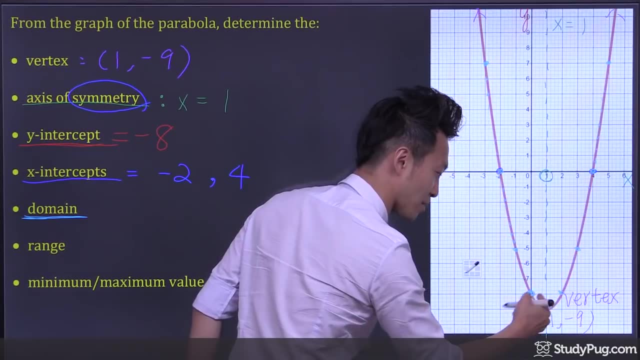 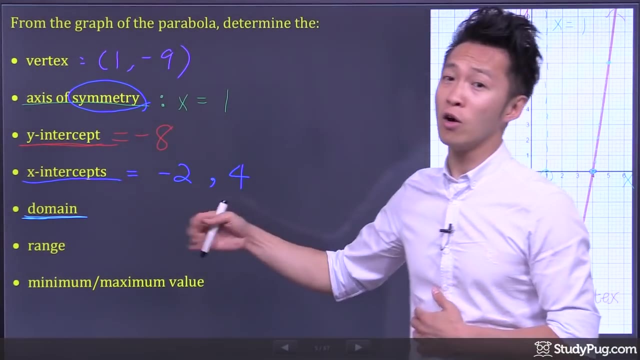 take on any negative values for x, And parabola can even take on 0 for x. That would be this point. See for the y-intercept. the x value is 0, right, So therefore the domain for a quadratic function is all real numbers And we. 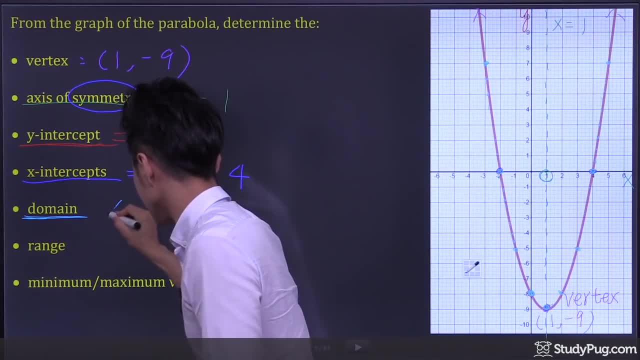 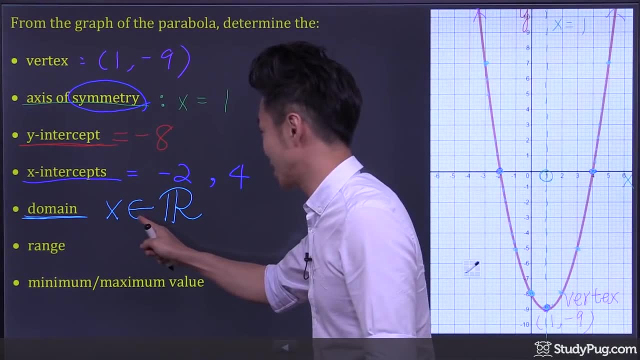 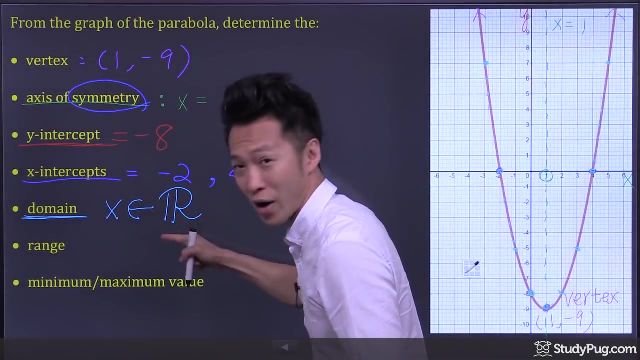 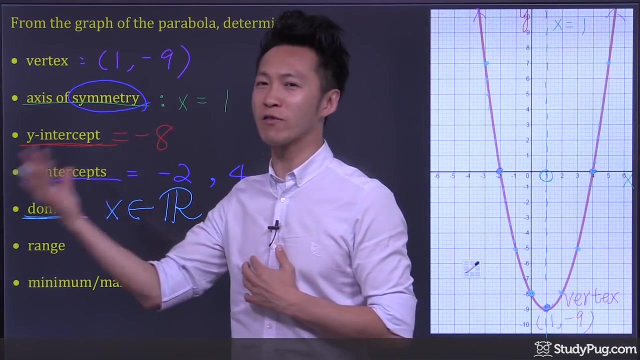 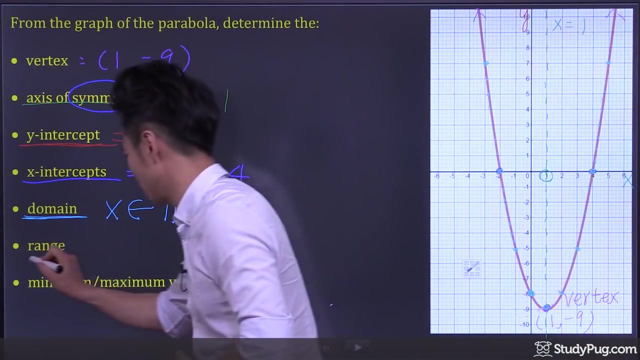 write a mathematical notation like this: x is all real numbers, All real numbers. This symbol means is, And this symbol here represents: see this symbol here is a r with an extra bar. represents all real numbers. In fact, the domain for any quadratic function is always: x is all real numbers. Next range: 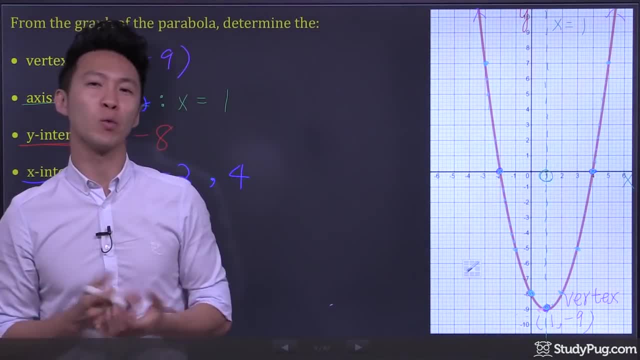 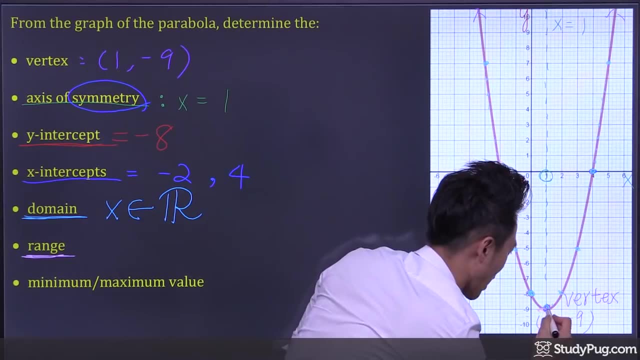 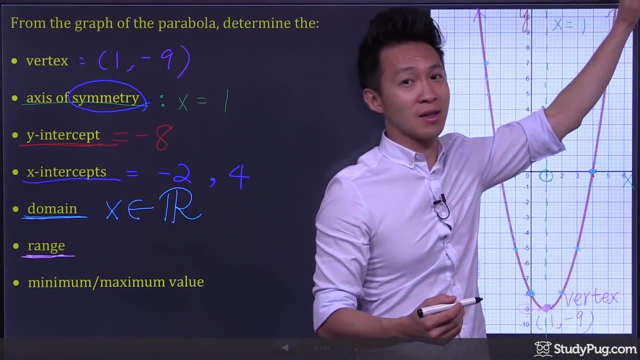 By definition, range is the set of y values for which a function is defined. So here the parabola only go as low as right, here, where the y value is negative 9. However, it will go as high as it likes, And therefore we say: 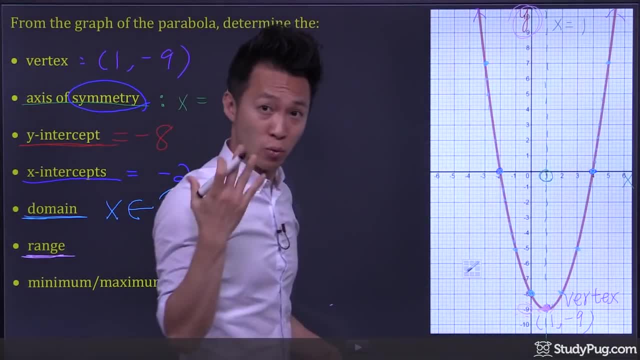 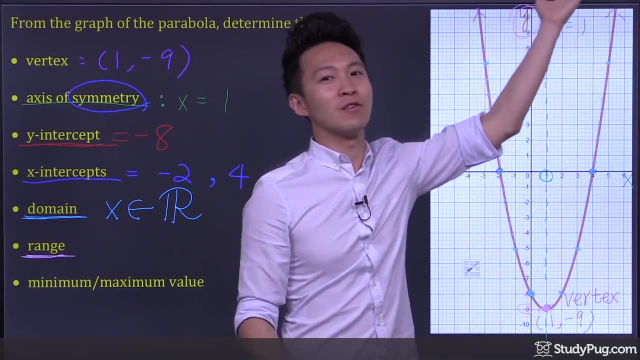 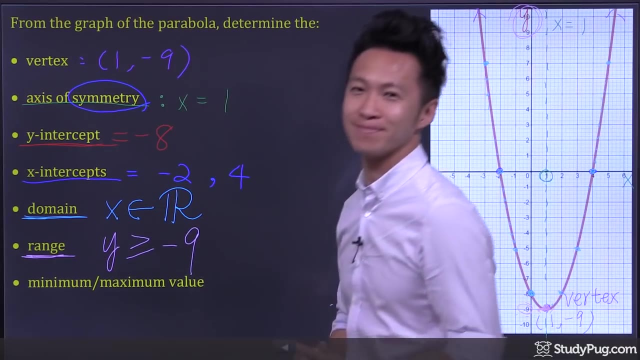 the range range talks about y, right. So the range is y must be negative 9 and anything above. So the range is y is greater than 0.. So the range is y is greater than or equal to negative 9.. Does this parabola have a minimum value or a? 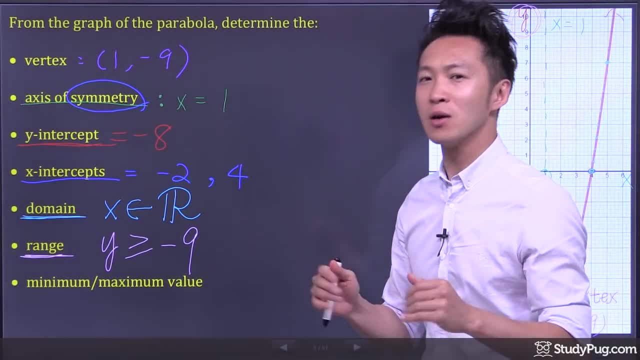 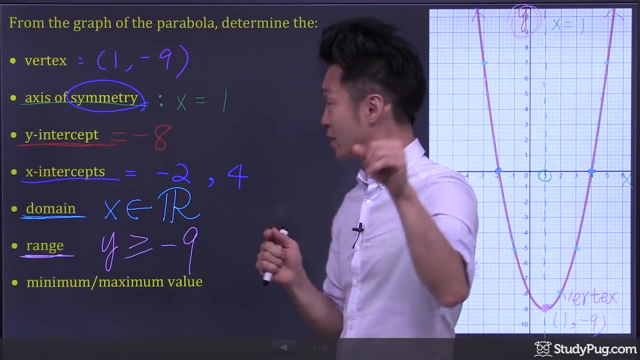 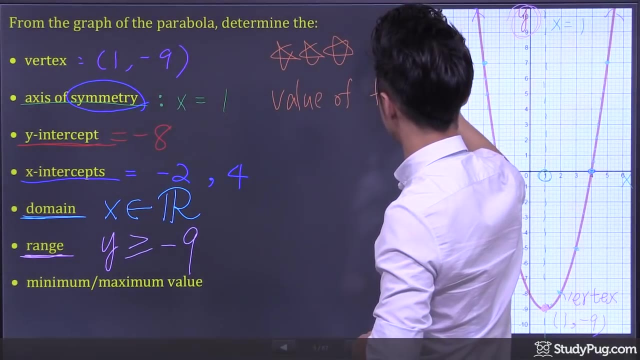 maximum value. Well, first of all, in math, whenever we talk about the value of a function, we are always referring to the y-value. Remember that Value of a function always refers to a value. So remember, all values are equal to a function. So that's how the function is. 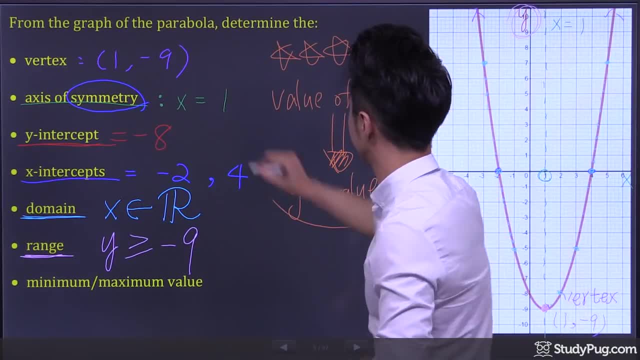 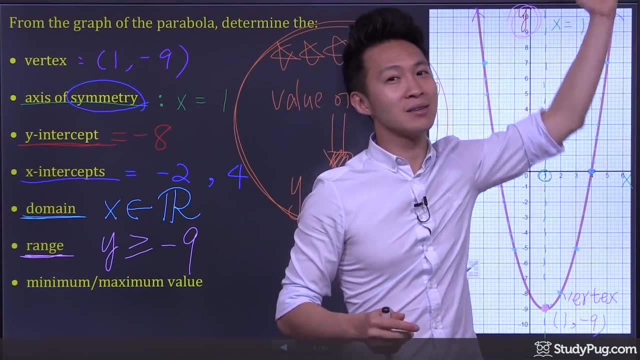 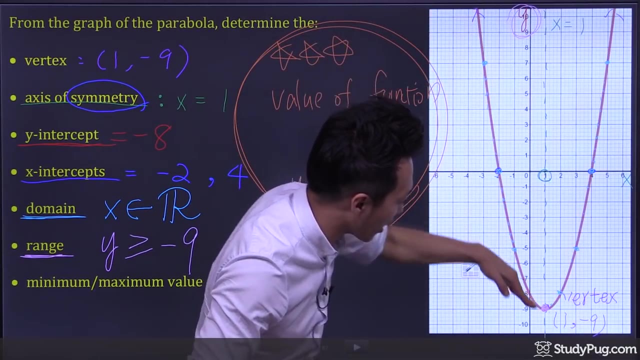 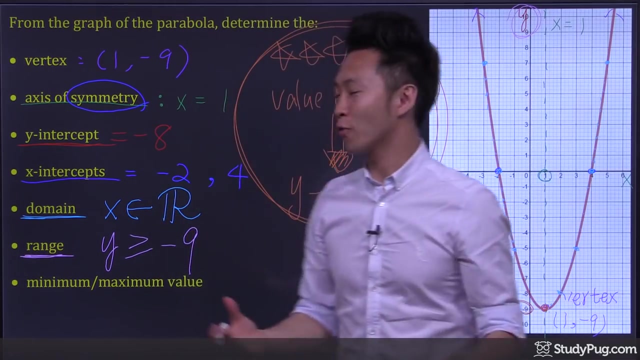 to the y value. Now, since the parabola can go as high as it likes, there's no maximum value. However, parabola can only go as low as right here, where the y value is negative 9. Therefore, 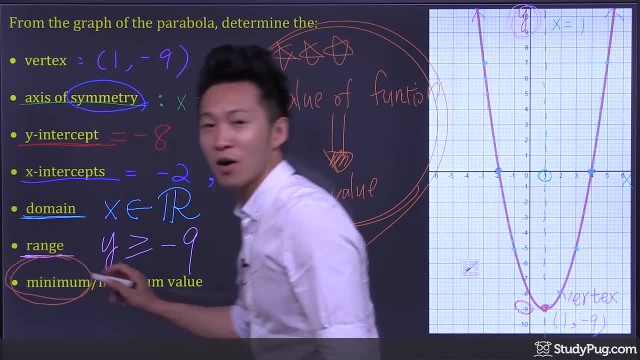 we say this parabola has a minimum value of negative 9..